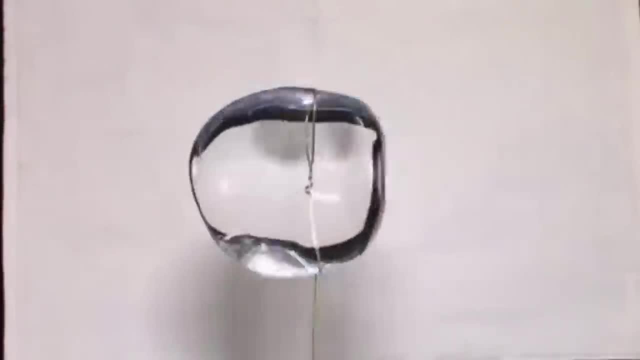 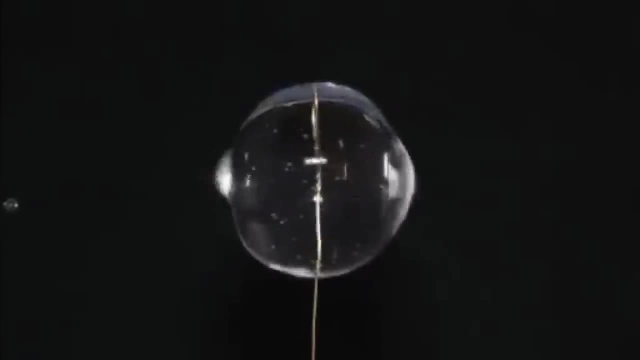 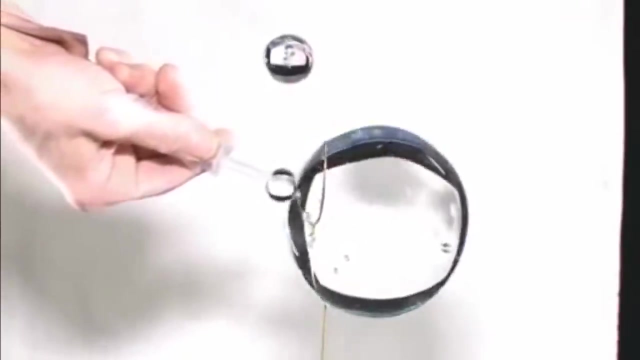 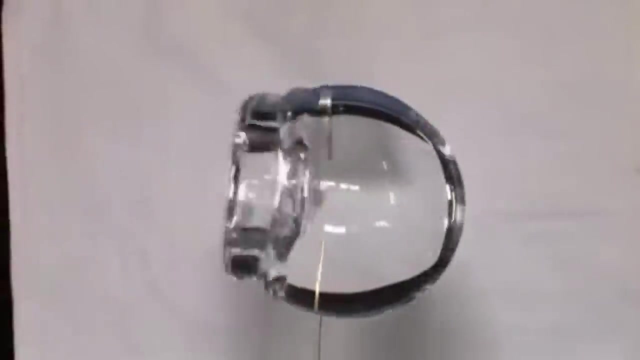 Okay, This is what you do: A black background. Yeah, So that's about 800 mils. So this should put it around 1100 milliliters. Let's see what happens here. Okay, Okay, Okay, Oh, I just love that. Look at that Amazing. 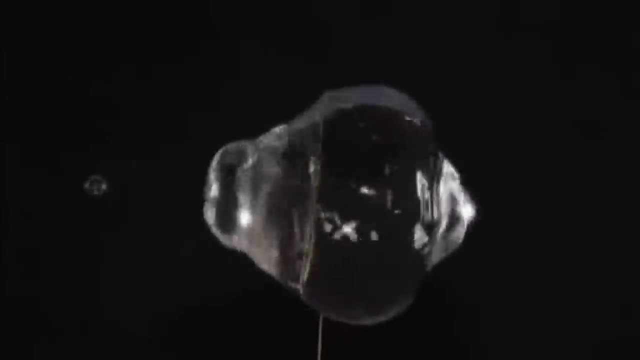 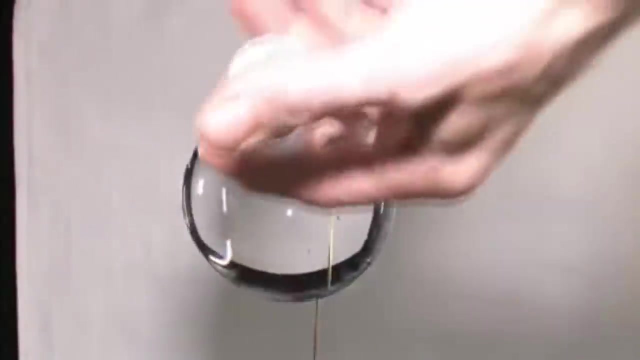 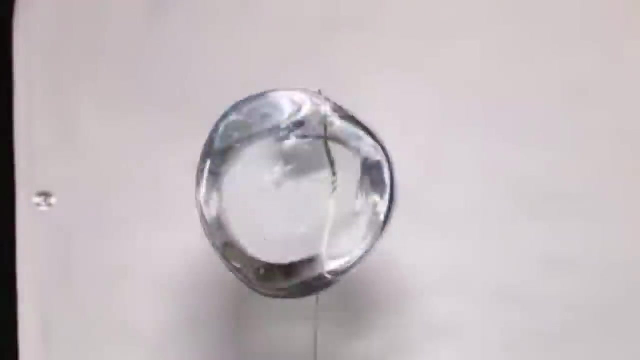 Just one of these jaw dropping moments. Okay, Here we go to do it again. Looking into the camera, Big puff, Here we go. Oh, right at the lens. I saved the lens. What I'm planning to do is, after this whole series of experiments, 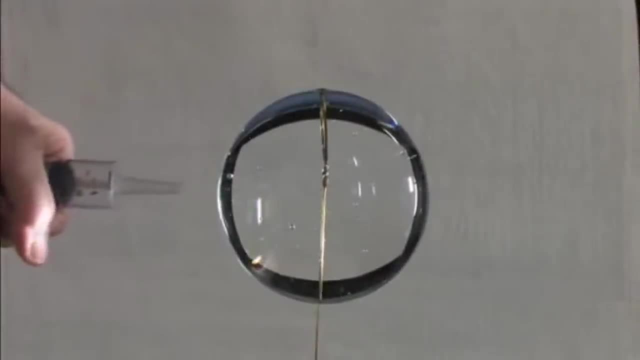 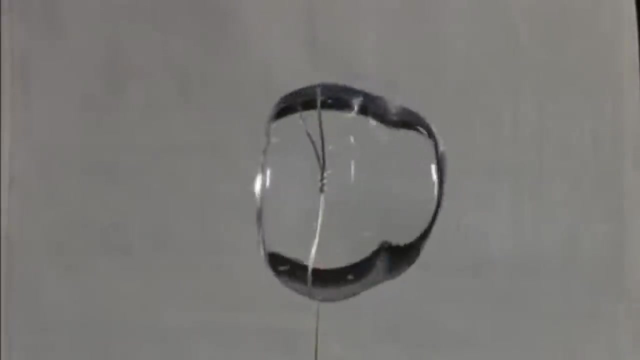 I'll suck all this water up with a syringe, I'll put it back in bags and I'll use it to make tea with. So I'll end up drinking my experiment. You got to conserve your resources. when you're in a frontier, You don't get to see this. 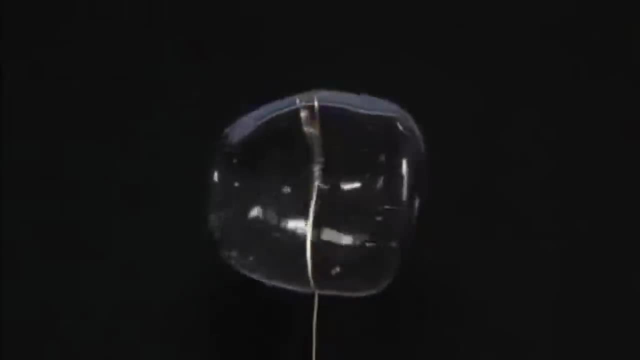 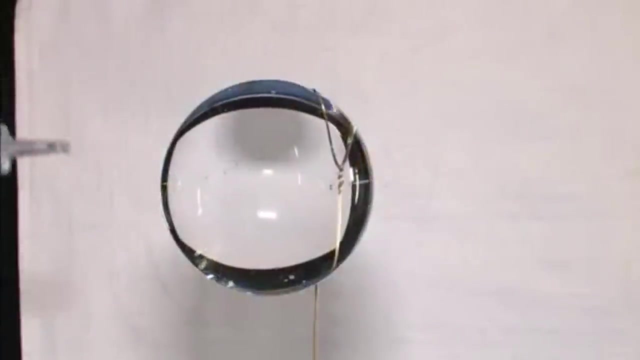 as common intuitive observables on earth, And so when we go into a frontier, our normal earth home intuition no longer applies to this. This rule works. Next, I can't, And instead of putting a puff of air on it, I'm going to put a puff of water. This is going to have a lot more momentum in it than the air. 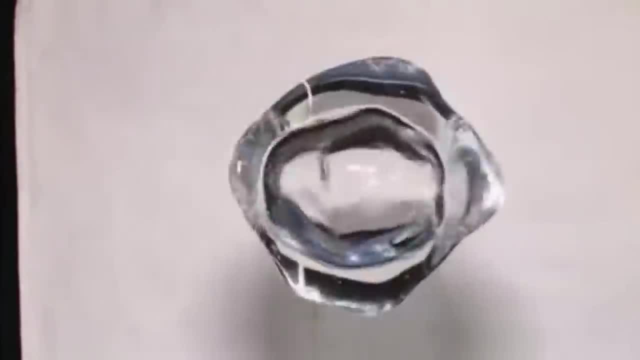 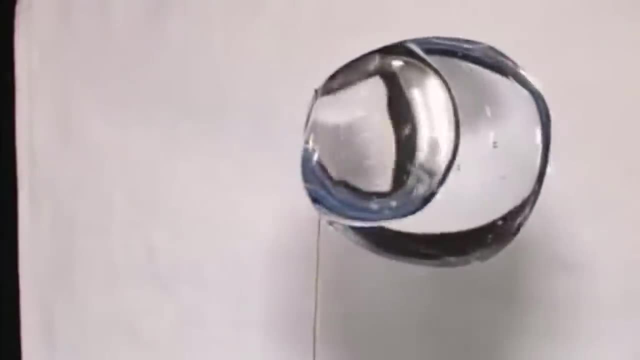 Whoa, Whoa. I was afraid. Oh, look at that Cool. I squirted water through. Oh, is it that cool? The water in the sphere went around the air cavity, formed a huge bubble, Wow, Wow. 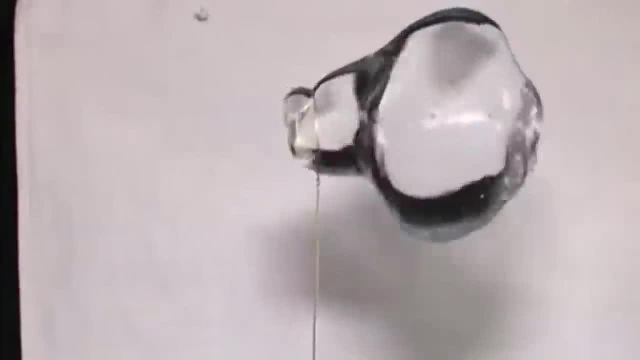 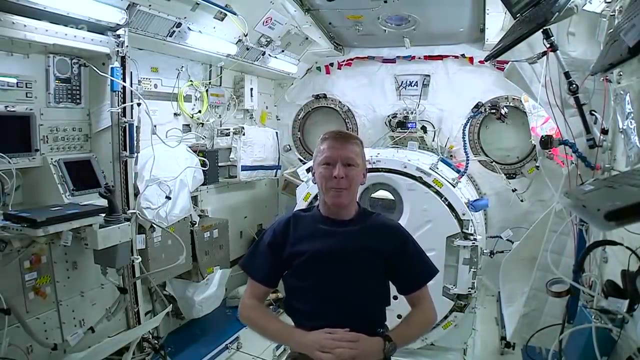 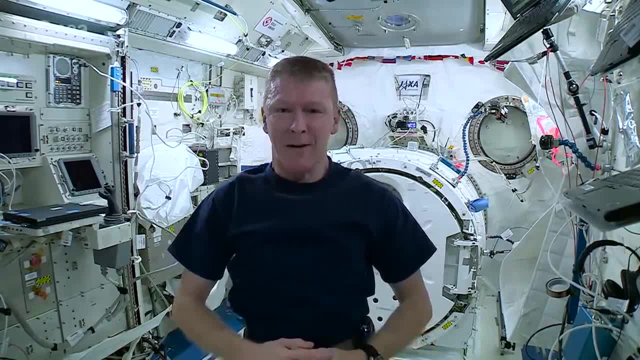 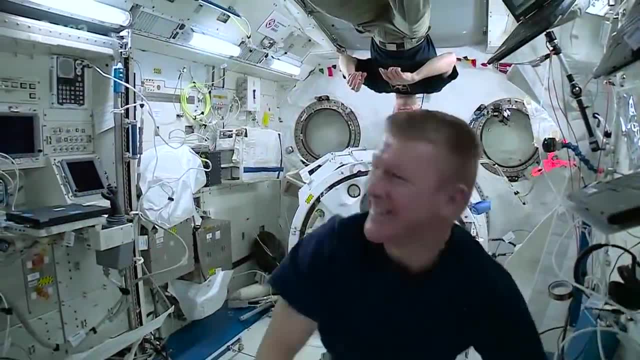 And does it make me feel unwell. So I'm gonna get Tim to spin me around doing something that would probably make me feel quite sick down on Earth. So let's see how that goes. This could be the worst idea I've ever had. 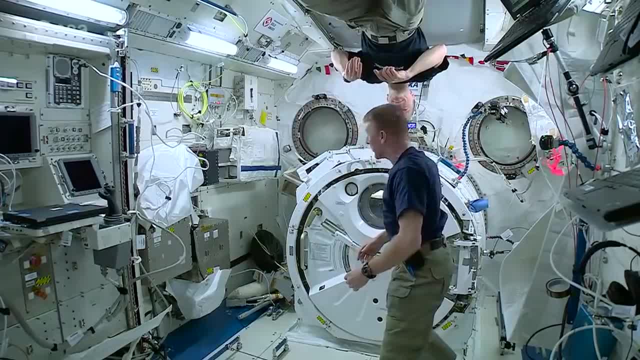 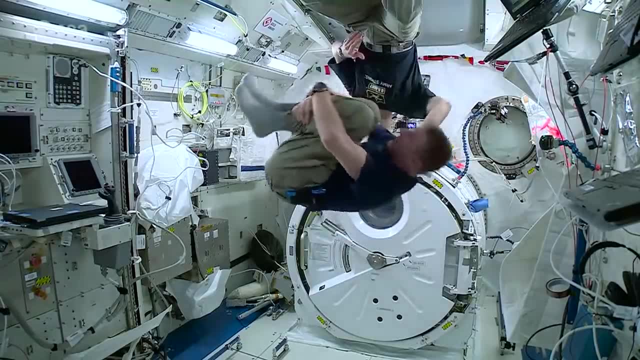 Oh, come on, you can do better than that, Okay. so yeah, I'll just go into a ball and start spinning And then, if you want to, just keep me go around, Yeah, yeah on axis, that's cool. 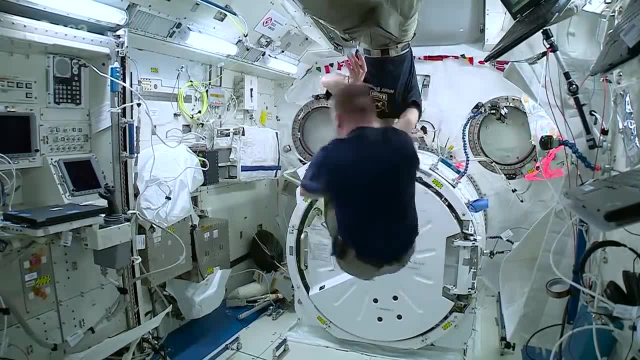 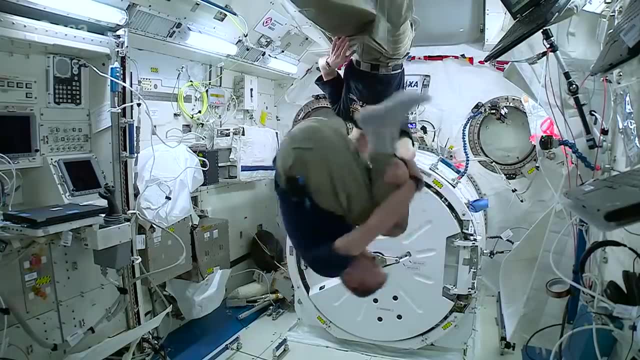 Actually, it's more provocative when you go off axis. Yeah, but I can't even control it. Yeah, no, don't worry, Provocative's fine, Just keep it going. Do I go faster? Yeah, Let's go for it. 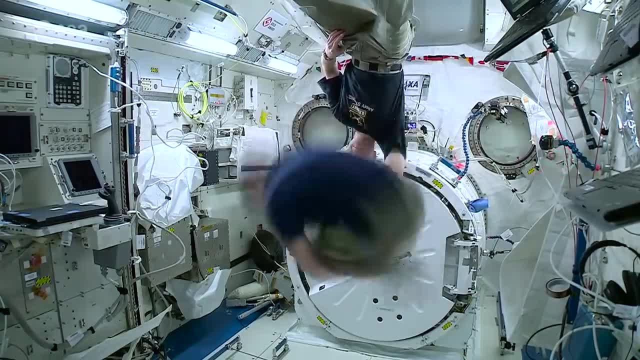 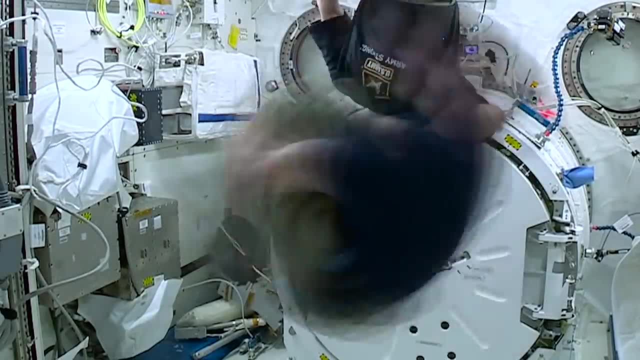 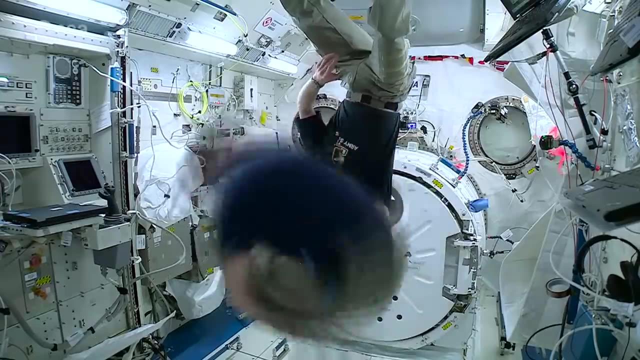 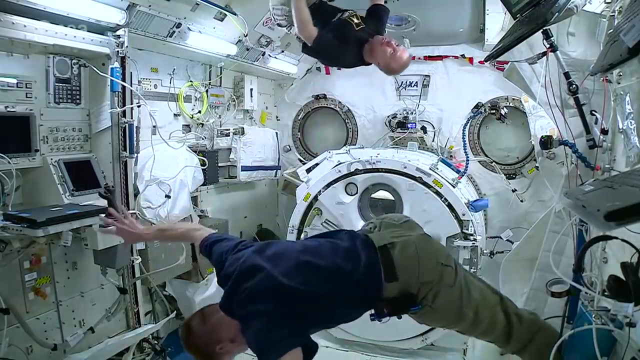 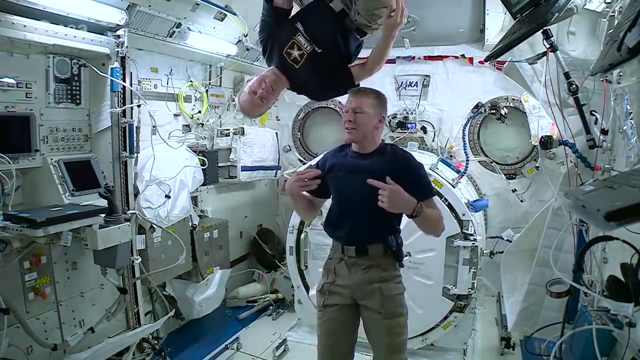 That's good. Okay, I'll see if I can. I'm feeling dizzy. I'll see how quickly it stops. So it definitely felt dizzy. I was a bit dizzy initially and now it's gone. No, is that quick. 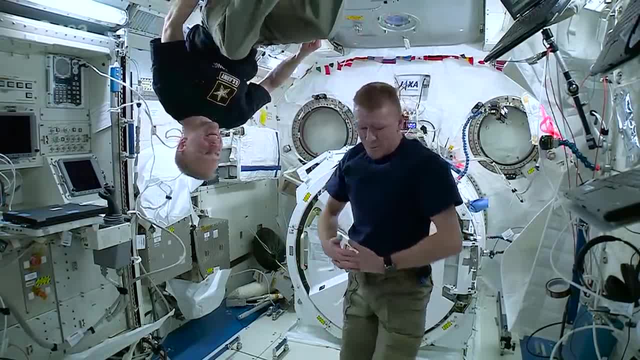 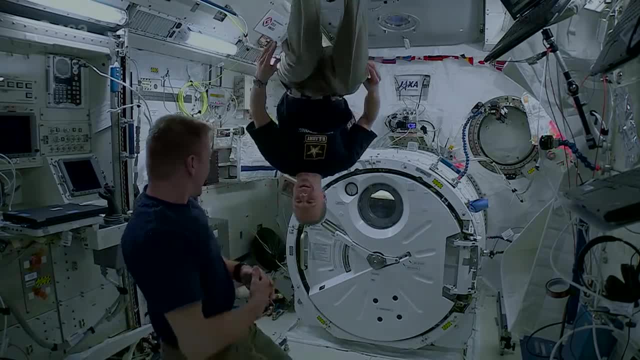 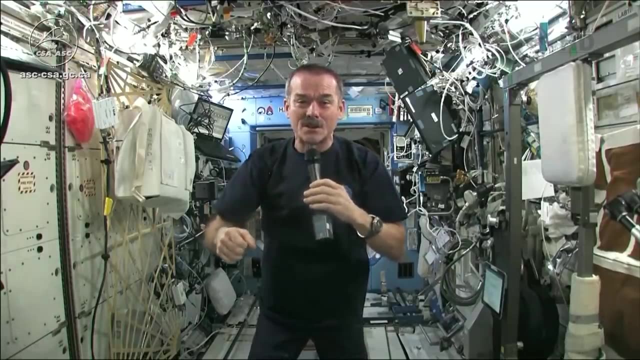 Yeah, completely normal, Amazing. Yeah, and again, I wouldn't be able to kind of just get off a fairground ride spinning that quickly for so long I feel normal. Yeah, Crazy, It is amazing. Number two Students from Nova Scotia ask Chris Hadfield to wring out water from a cloth. 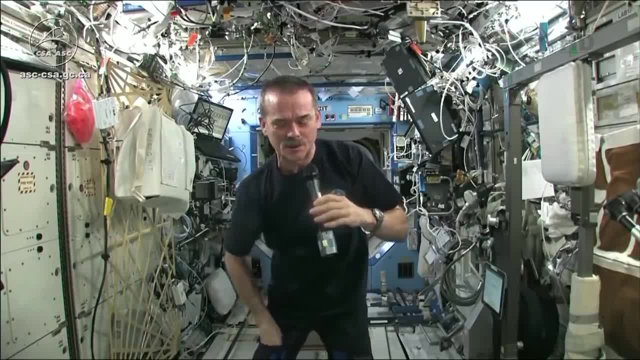 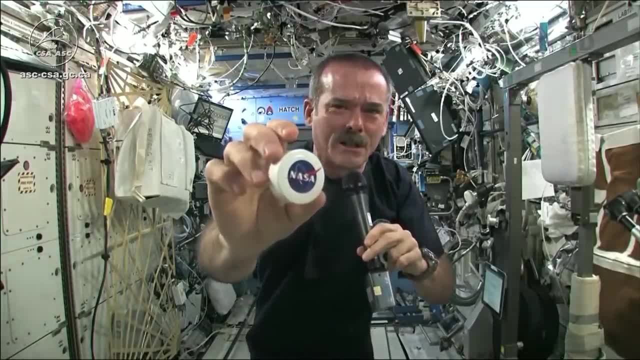 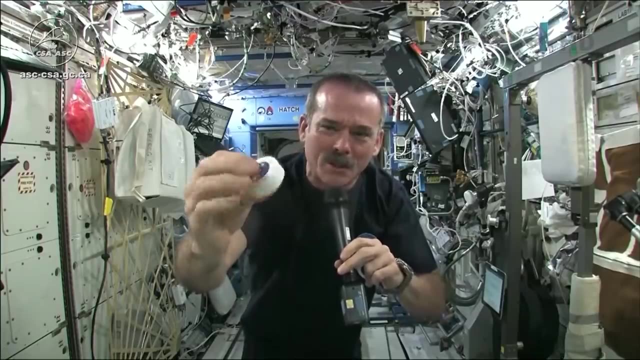 The results are unexpectedly quite interesting. We might have the coolest washcloths ever here on the space station. I'm going to show you. Here's one of our washcloths And it's packed, It's put down into this little tiny hockey puck so that it saves space. 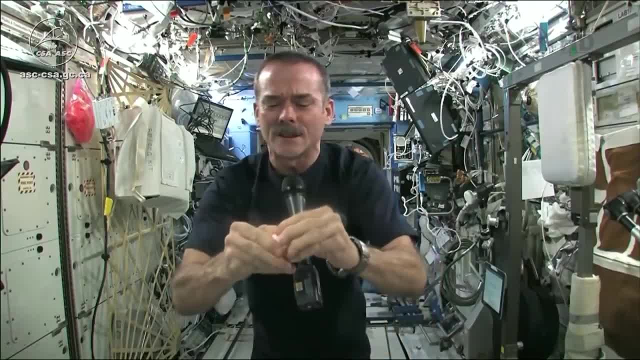 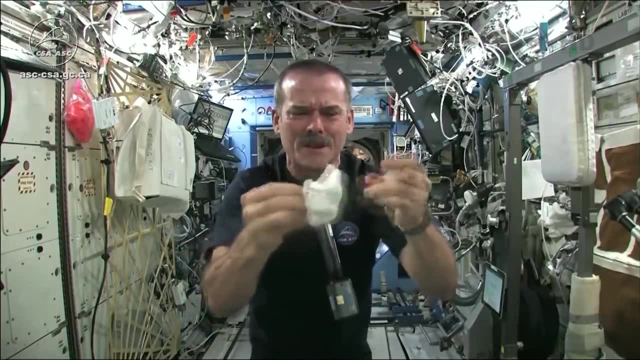 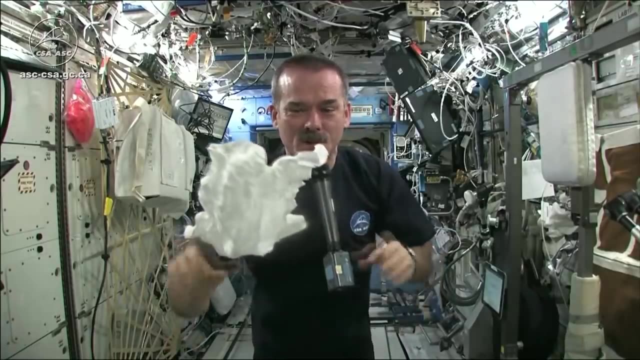 But when you open up a hockey puck, and so when you open up your hockey puck and turn it into a washcloth, it was compressed in a great big vice somewhere. Okay, So here's my washcloth, Like a magic trick, And now I'm going to get this soaking wet and then we're going to see what'll happen. 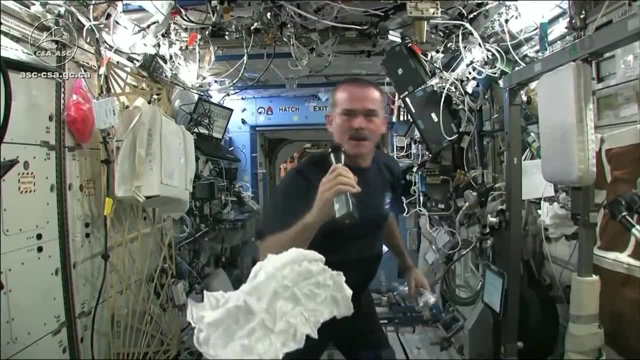 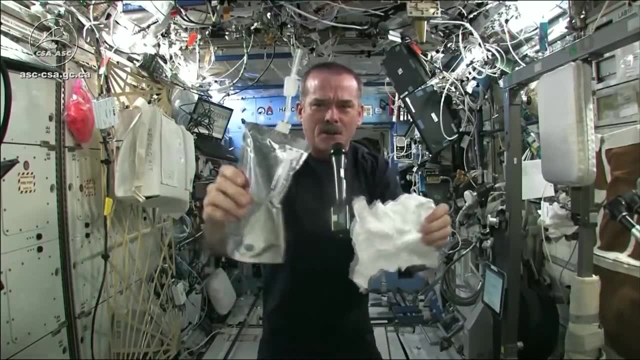 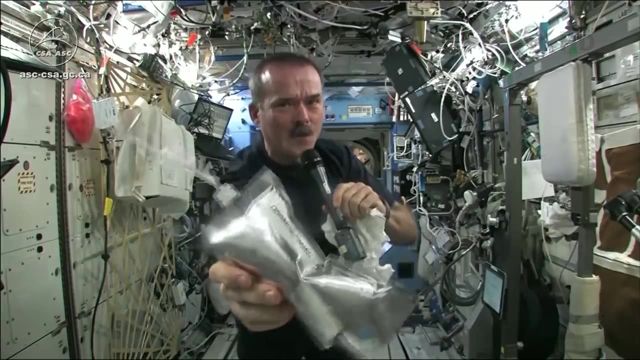 when we wring it out. Meredith and Kendra suggested that I dip this in a bag, but bags don't hold water in space, So instead I filled a water bag. This has drinking water in it, And I'm going to squirt a bunch of water into this washcloth. 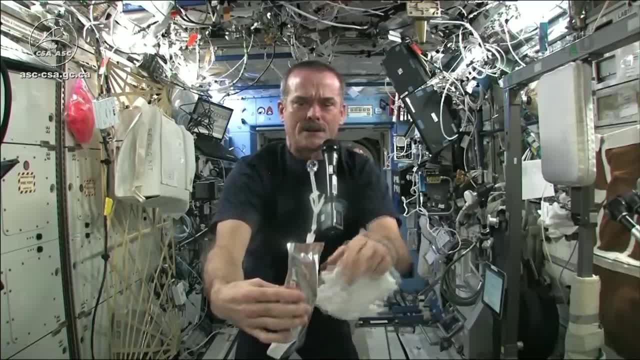 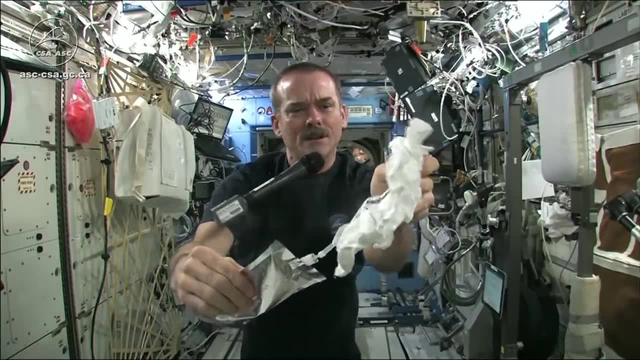 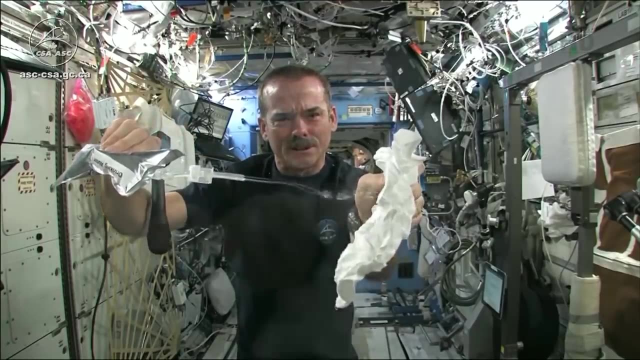 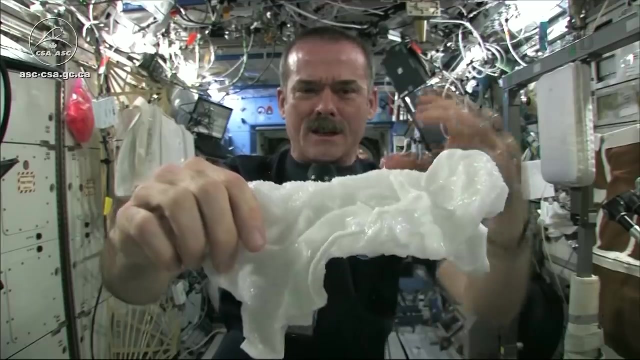 Okay, So here's my washcloth. Let's take a look at that. Okay, So here's a soaking wet washcloth. Get the microphone so you can hear me while I'm talking. And now let's start wringing it out. 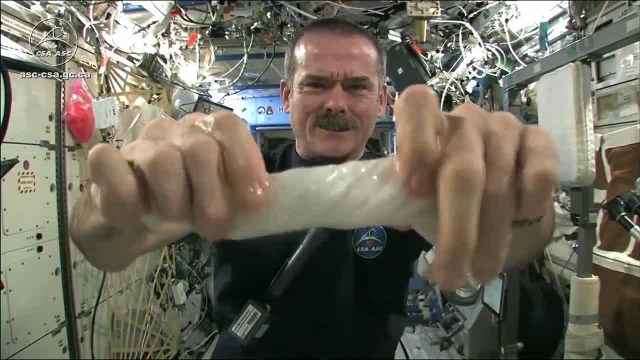 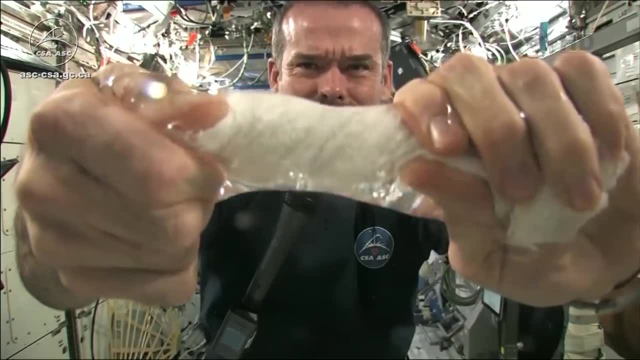 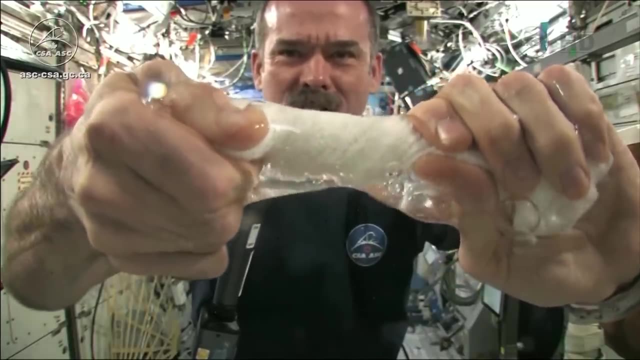 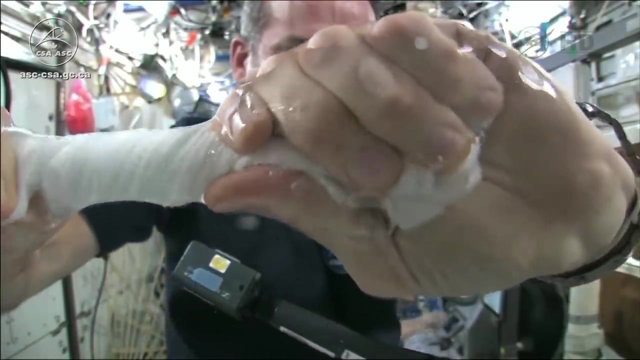 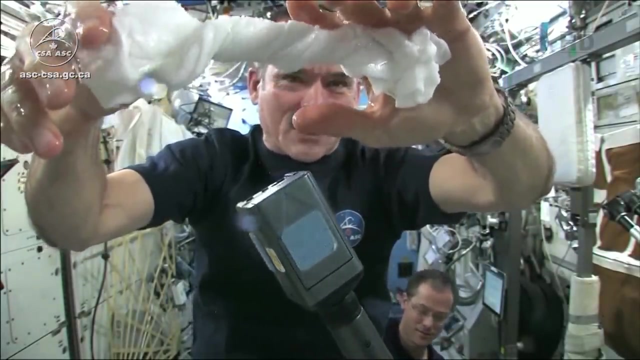 It's really wet. It's really wet, it's becoming a tube of water. the water is all over my hands. in fact it rings out of the cloth into my hands and if I let go of the cloth carefully, the water sort of has it stick to my hand. 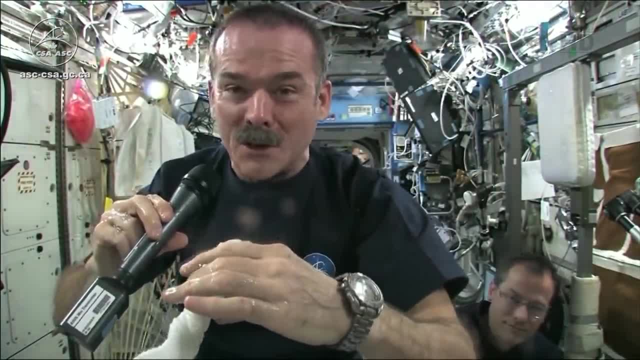 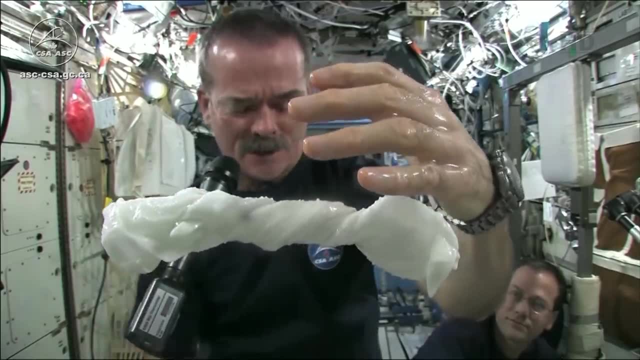 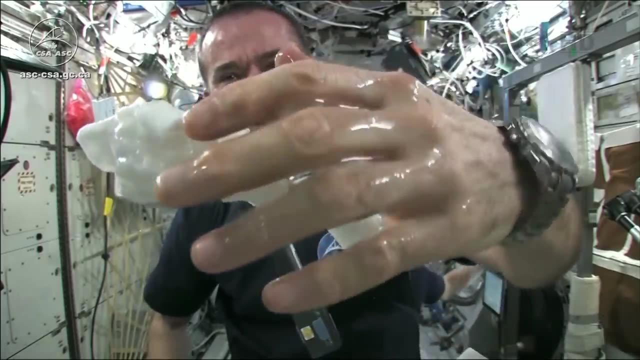 okay, so the experiment worked beautifully? and the answer to the question is: the water squeezes out of the cloth and then, because of the surface tension of the water, it actually runs along the surface of the cloth and then up into my hand, almost like you had jello on your hands. 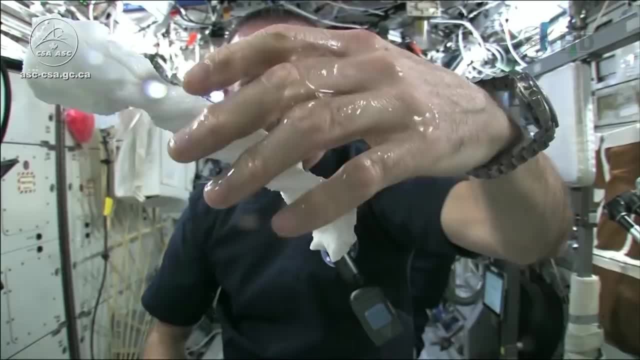 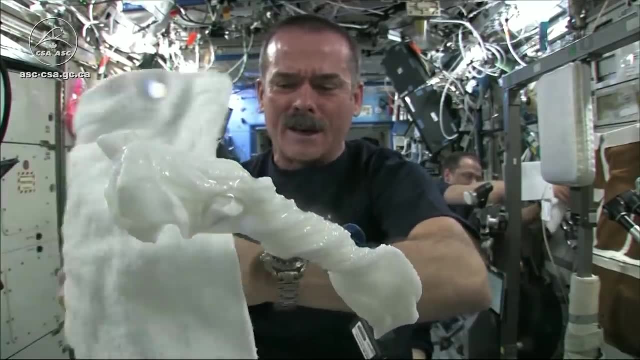 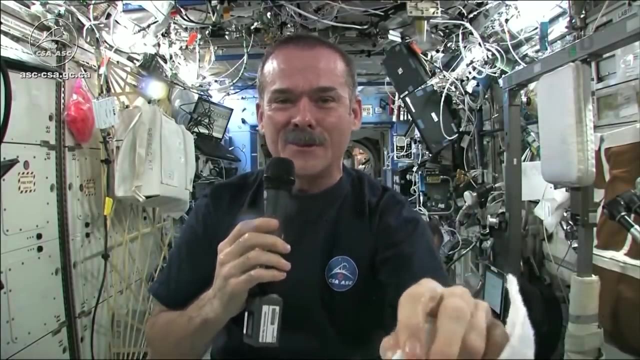 or gel on your hand and it'll just stay there. wonderful, wonderful, wonderful moisturizer on my hands and the cloth doesn't really unravel itself, it just stays there, floating like a, like a dog's chew toy, soaking wet. great experiment, worked perfectly. Meredith and Kendra congratulations. 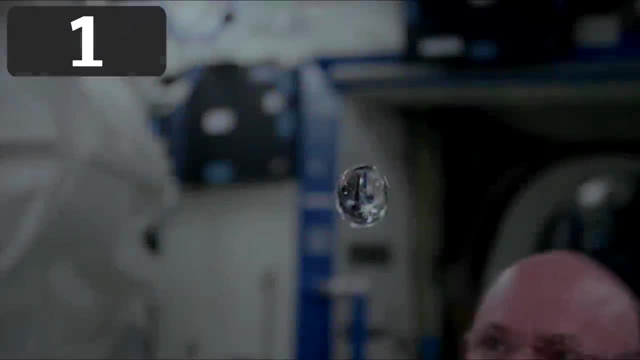 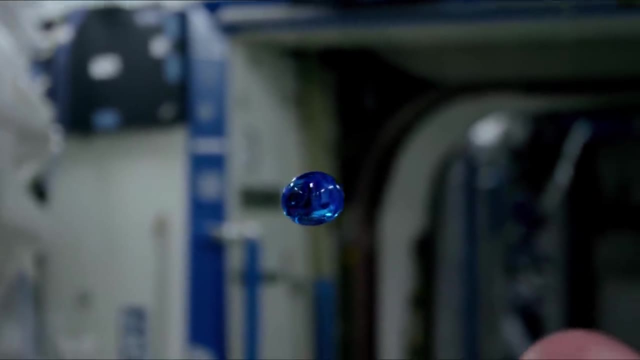 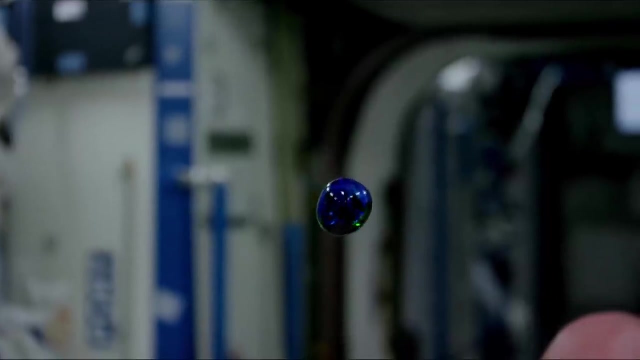 great idea, so this has to be number one. US astronaut Scott Kelly tests how various dyes interact with a floating ball of water. it's almost like he's creating a miniature planet. he's drawing her. Oh, this was the first time I saw a silicone lipid. 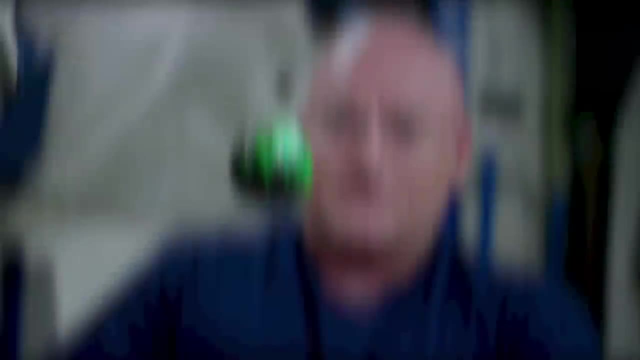 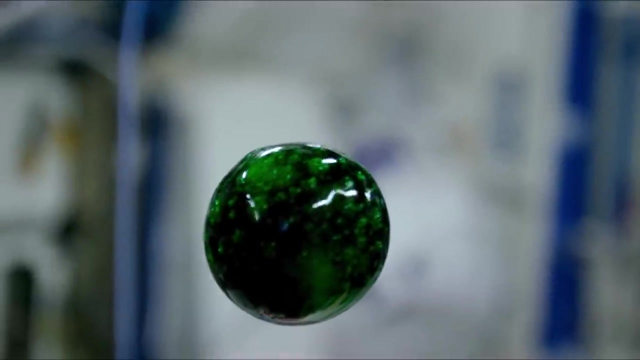 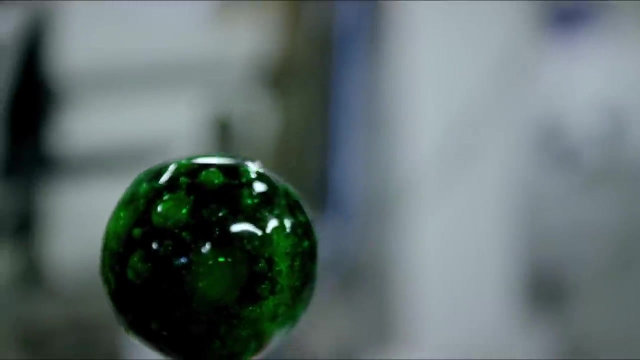 in a water bottle. I was really confused. I was really confused. he was forcing the ball around and it's going super clunky. okay, I'll just gently equipped him like a glove. it felt like he was using a Beverley like feeling really more of like my那 u.